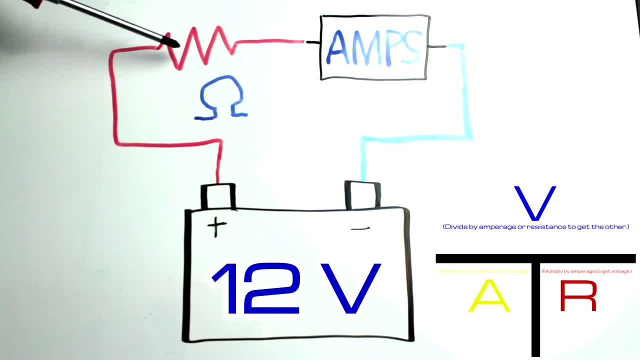 volts pushing through our circuit, We get to a resistor. It is a two ohm resistor. Now, if we have two ohms and 12 volts, we're going to end up with six amps. Amps is our current flow, Two ohms. 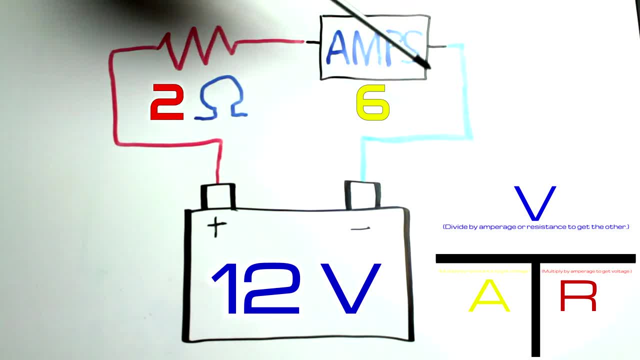 is not a lot of resistance. current can flow through here pretty freely. So again, if we have 12 volts of push through two ohms of resistance, you end up with six amps of current flow. How about we double the resistance and see what happens? then? We're going to stick with our 12 volt battery and with four ohms of. 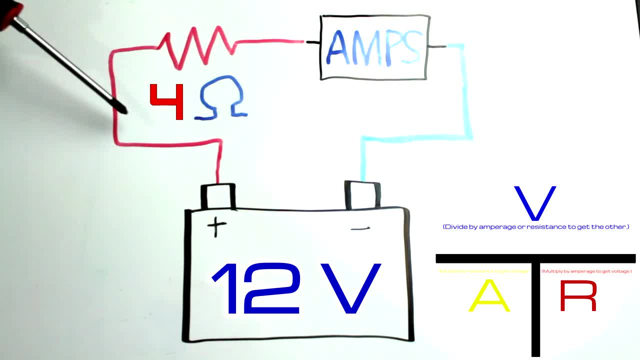 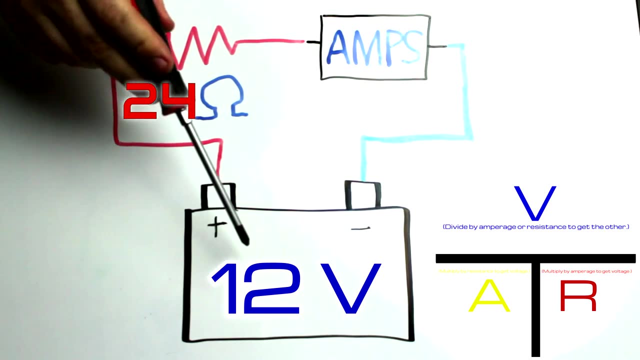 resistance. it's resisting more, so current can't flow through here as freely. You end up with three amps. You may notice that we doubled our resistance, so the amperage was cut in half. How about we raise this resistor rating to something really high like 24 ohms? So we have this 12 volt push. 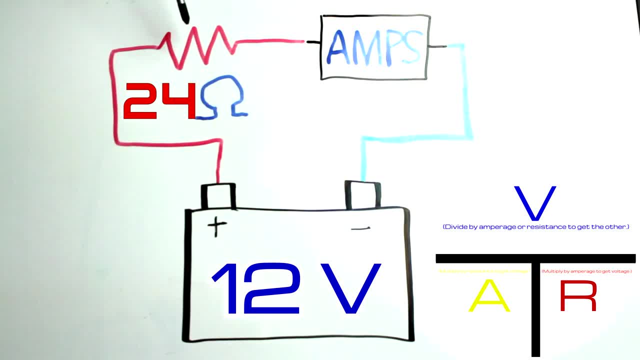 through this 24 ohm resistor and it resists a lot, so we're not going to have a whole lot of current left over. So, doing the math, 12 divided into 24 parts is going to be one half. We've got 24 ohms. 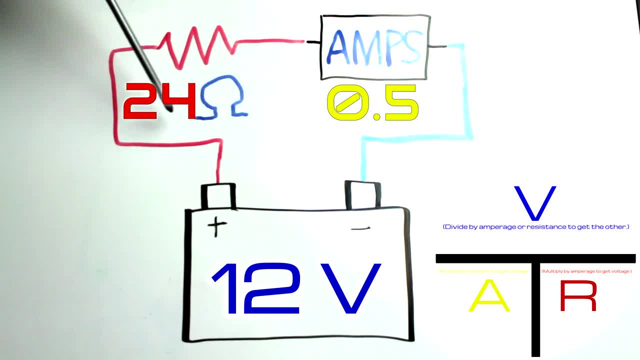 of resistance holding back our 12 volts here, so only half an amp goes through this circuit. And one last one: what if we had a really low resistance here, 0.5 ohms? Well, 12 volts comes along and hardly anything is holding it back, so it's going to flow right. 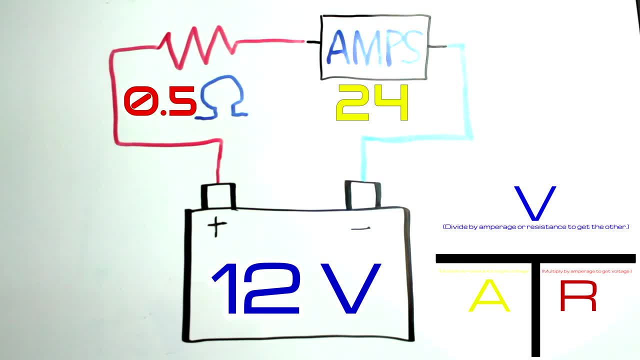 through there real fast. That'll be 24 amps of current flow, to be precise. If you had a 20 amp fuse on your circuit right there, that would blow it out. How else could we use ohm's law? Well, if you knew your resistance and your amperage, you could figure out your voltage. So if you have 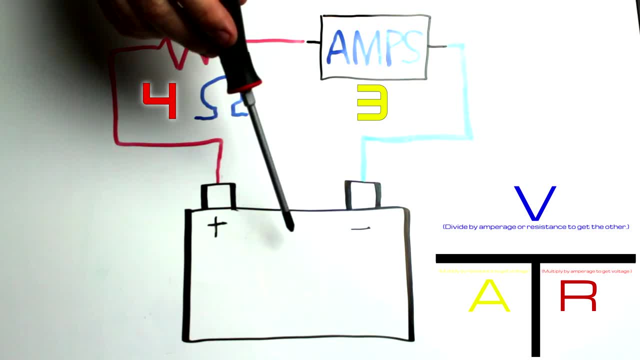 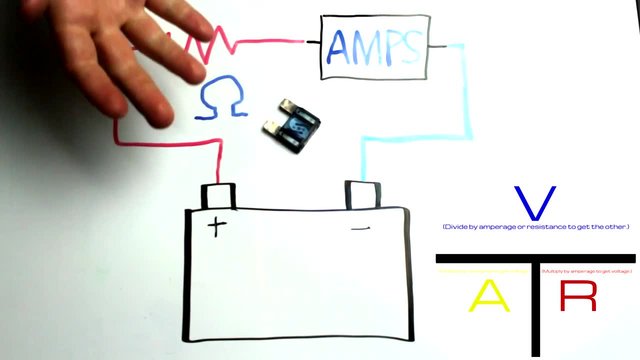 four ohms and three amps. you can multiply these two to get your voltage. Four times three is 12.. If you'd like to learn more about fuses, I'll provide a link to my video about them If you enjoyed this lesson. there's a whole lot more videos like this on my channel, so consider. 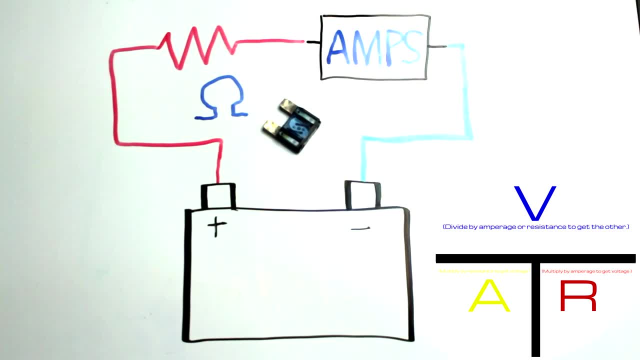 subscribing. At any rate, I hope you know more now than when you first clicked on the video. Thanks for watching and I'll see you in the next car. simplified video.